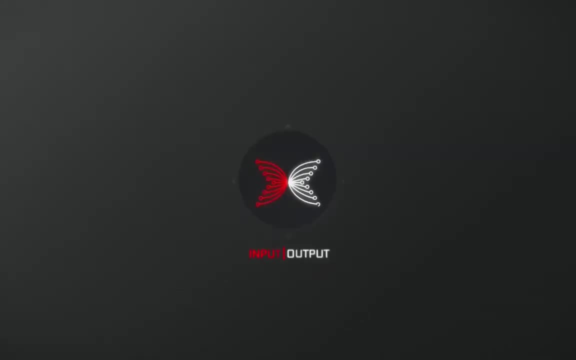 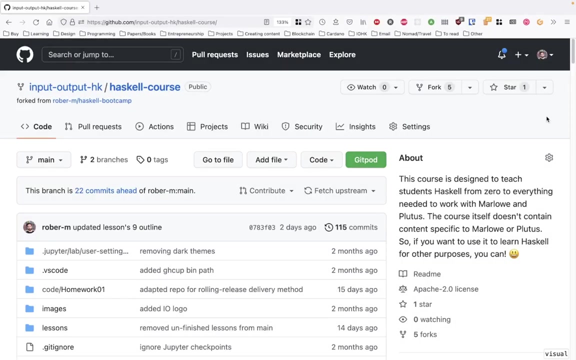 Welcome to the first lesson of the Input-Output Haskell course. Today we will look at how to use the resources, then we will go over an introduction to Haskell and finally I will show you how you can complete the homework. So this is the repo: input-output-hk-haskell-course. 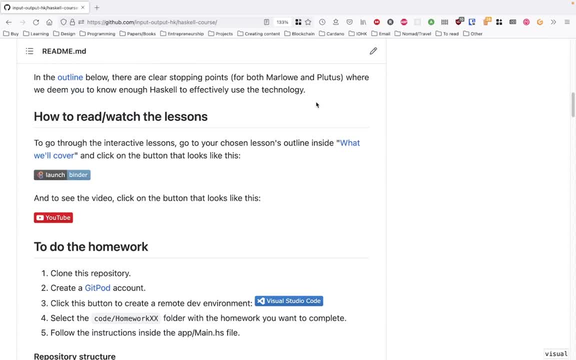 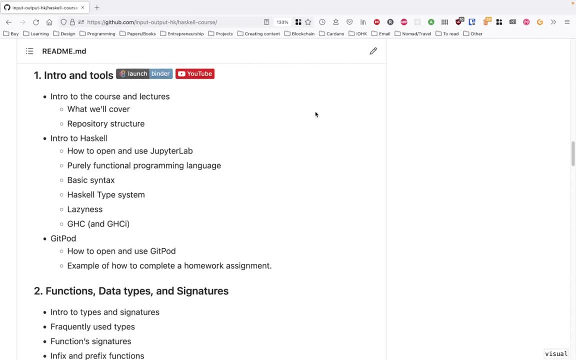 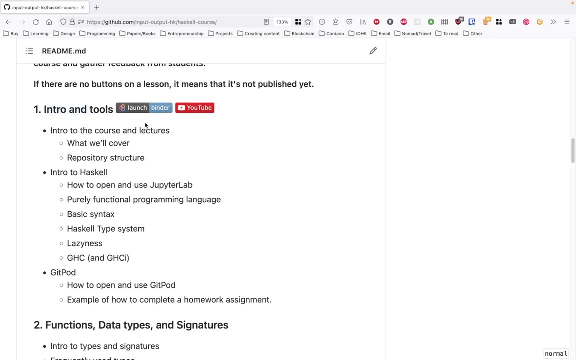 and if you scroll to the readme you will find detailed instructions of how to go through the course. But it's really easy. all you have to do is go to the outline and right after each lesson's name there will be two buttons: The launch binder button to open. 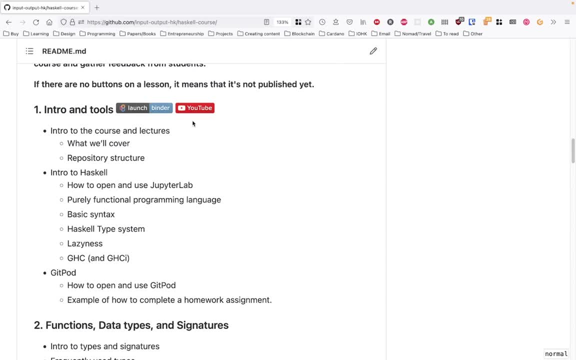 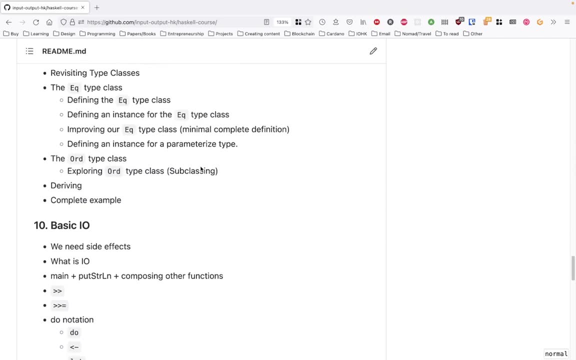 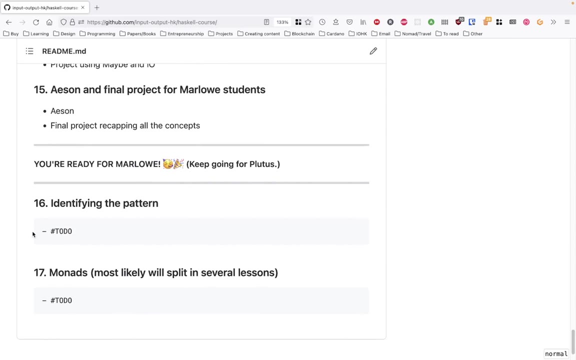 the interactive lesson and the YouTube button to watch the video lecture. You may notice that not all the lessons will have the buttons. That's because they haven't been published yet. But if you keep scrolling you'll encounter stopping points when everything needed to. 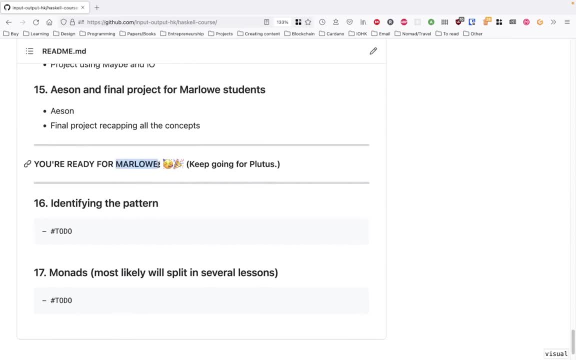 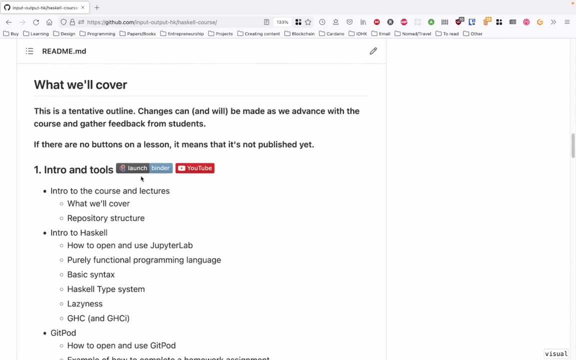 use a certain technology- Marlowe in this case- has been covered. So if your objective was to use Marlowe, you're good to go. Else, you can keep going. Ok, so let's open the first interactive lesson. 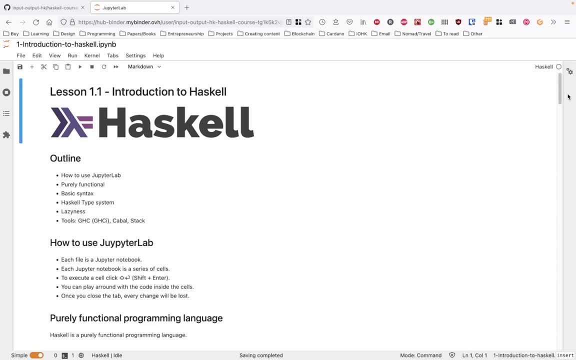 Ok, so after waiting for a little bit, our interactive lesson will open. This is a Jupyter lab. There's a lot of things going on here, but you're here to learn Haskell, and for that you don't need to know much about Jupyter. The entire file is the lecture You can read. 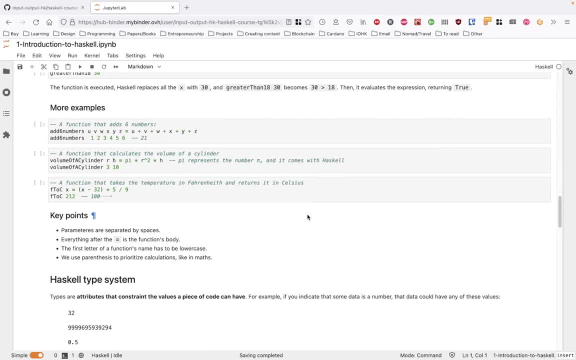 it like any other text-based content, But the good thing about it is that we can run Haskell code inside it. For example, this is a Markdown cell and this is a Code cell. If we select a Code cell and type in the code cell, we can see that it will be a code cell. 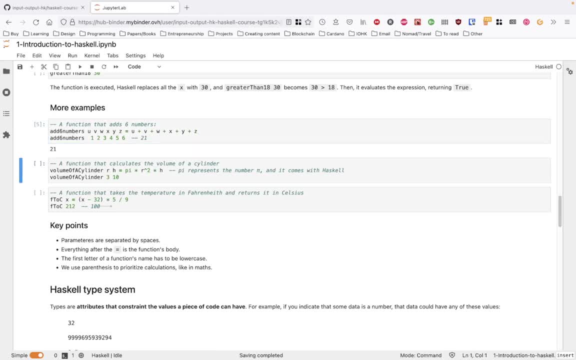 If we select a code cell and type shift enter, Jupyter will compile and run the code for us and show the result below the cell. Also, you're free to modify the contents and re-run the code as much as you want, Like this, But keep in mind that this environment is for 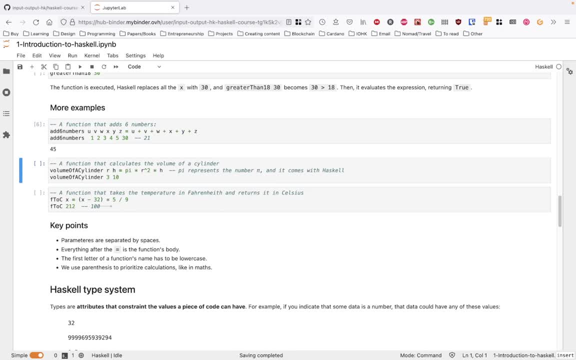 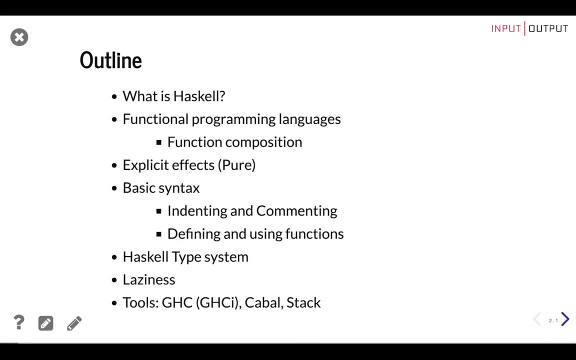 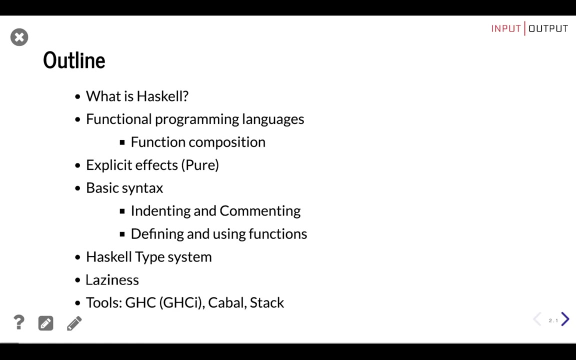 learning purposes. and once you close the tab, every change will be lost. Ok, we're ready for an introduction to Haskell. This is the outline. We'll start with functional programming, explicit effects, some basic syntax, Haskell type system and we'll finish by explaining why it's not always bad to be. 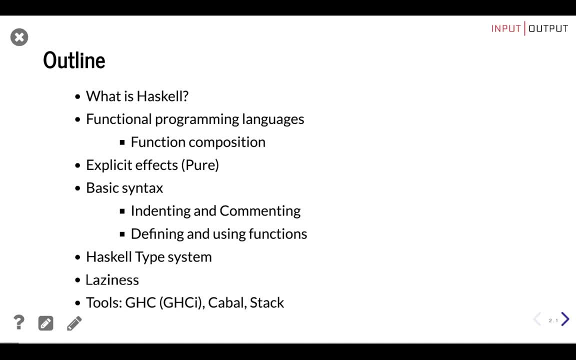 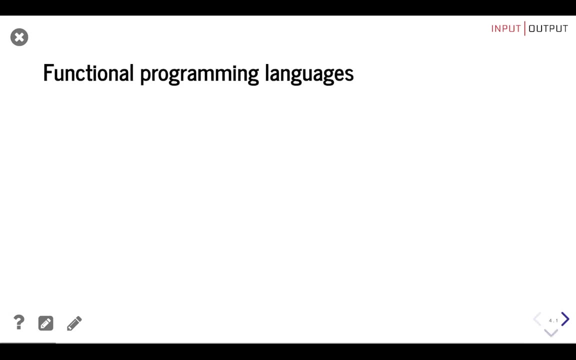 lazy. At the end I will name a few common tools, but only explain GHC. So what is Haskell? We'll go over each property of Haskell individually and answer this question at the end of the lecture. Haskell is a functional programming language. In functional programming languages function. 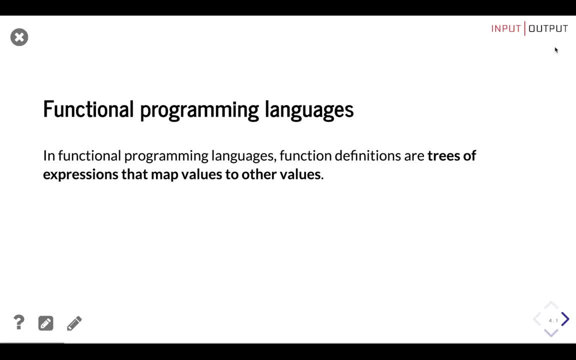 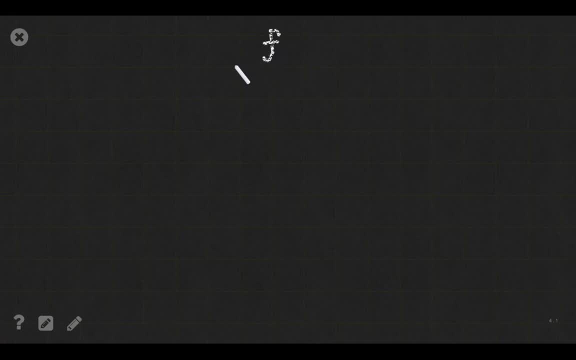 definitions are a tree of expressions that map values to other values. Let's unpack that. Okay, so functions are something that map values to other values. There are inputs and there outputs, so this something is a tree of expressions. so what's an expression? well, 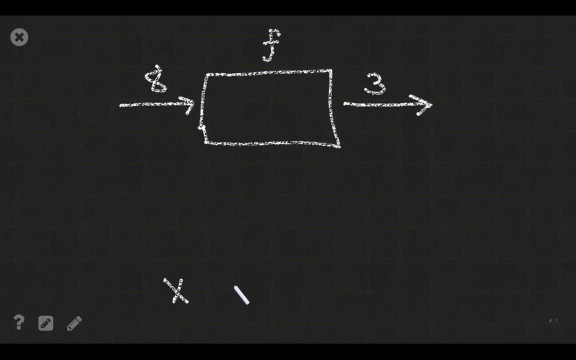 the variable x can be an expression, the operation plus can be an expression, the number one, the string hello- it's supposed to say hello. another function can be an expression, and we can combine this into more complex expressions. and then we can recombine them into even more complex expressions. 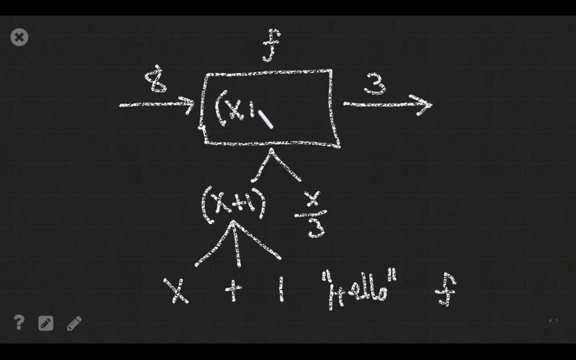 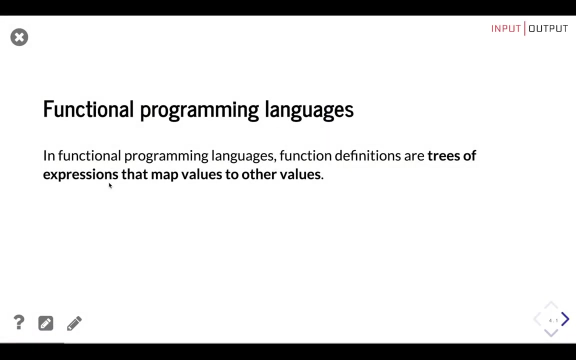 until we obtain the one we need. so that's it. functions are something that they makes an input and produces an output, and that something is a tree of expressions. okay, so what do we do with those functions? well, we create programs, and programs are constructed by applying and composing those functions. let's see what composing function means. so 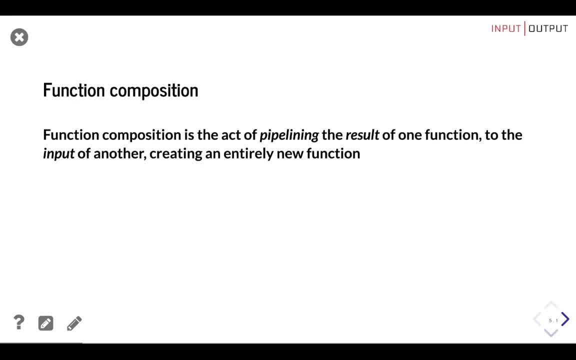 function composition is the act of pipelining the result of one function to the input of an output another, creating an entirely new function. like the usual function composition in mathematics, the result of each function is passed as the argument of the next and the result of the last. 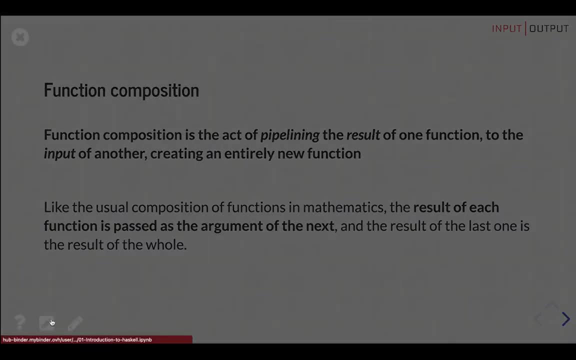 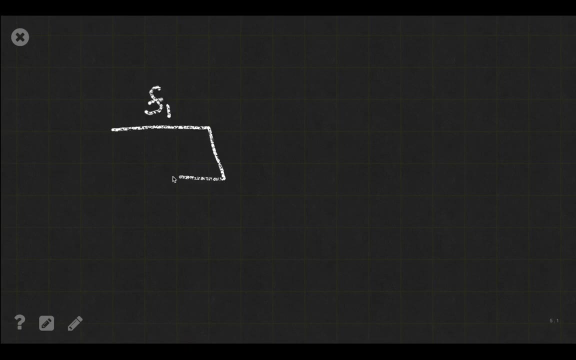 one is the result of the whole. so we have function one that takes an input, does something and produces an output, and we have function two that also takes an input, does something and produces an output. so function composition means that we take the output of the first function and we pass it as the input. 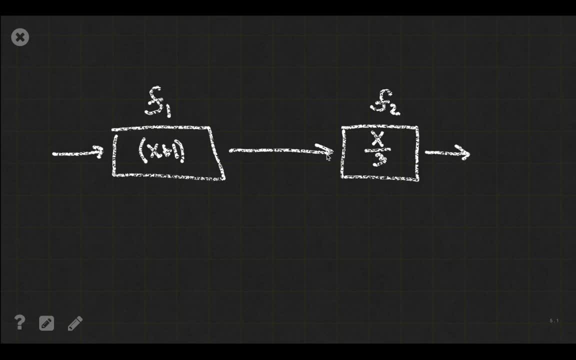 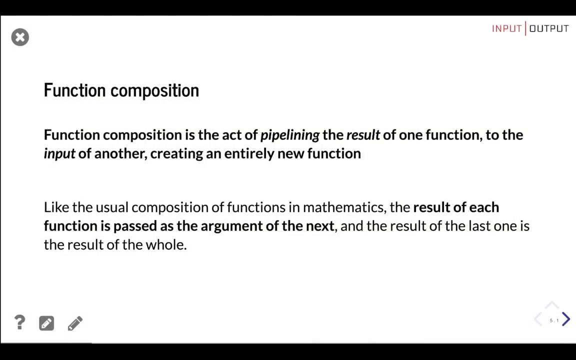 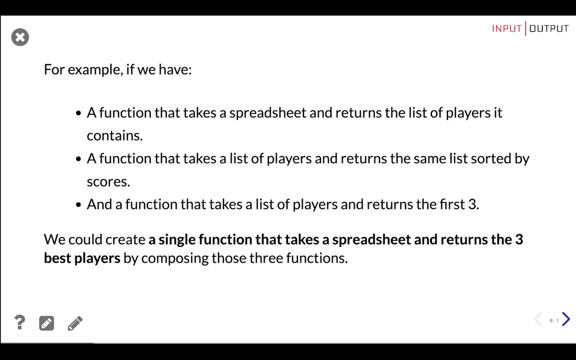 of the second one, thus creating a new function that takes an input- the same input as the first function, but a new function- and returns an output- the same output as the last one. So let's make it a little bit more concrete. For example, if we have a function that takes a spreadsheet and returns the list of players it contains, 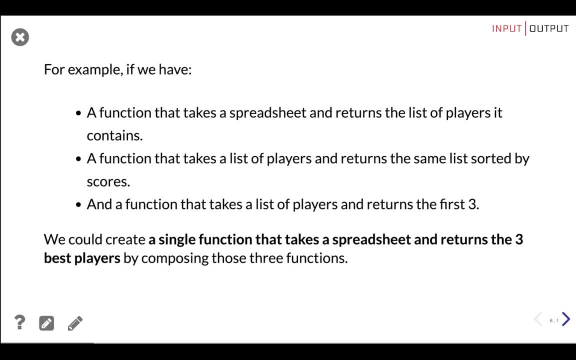 then another function that takes a list of players and returns the same list, but sorted by score, and the last function that takes a list of players and returns the first three. We could create a single function that takes a spreadsheet and returns the three best players by composing those three functions in the same order. I just described them. 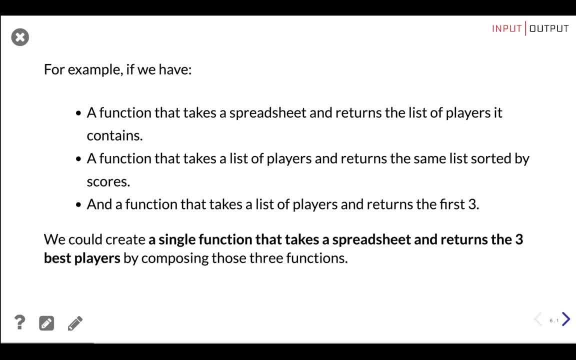 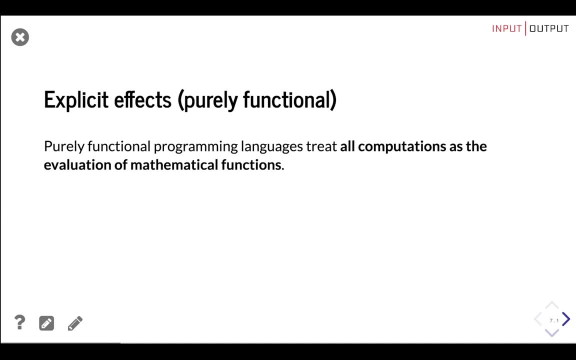 And that's it. That's all there is to it. But Haskell also has explicit side effects. Purely functional programming languages treat all computations as evaluation of mathematical functions. In mathematics, the expression y equals x plus one means that the value of y is a function that depends on x. 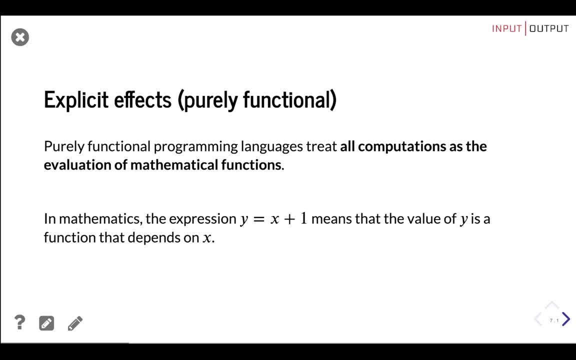 For a specific x, the value of y will always be the same, No matter if you are in Italy or in Spain, if it's 1994 or 2022, or if there are other equations in your notebook. y will care about the value of x and nothing else. 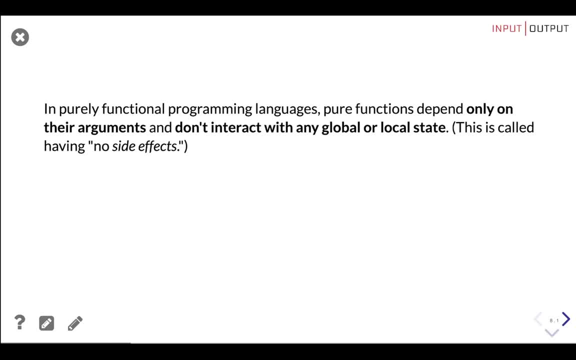 In purely functional programming languages. pure functions depend only on their argument and don't interact with any global or local state. This is called having no side effects. This means that for a specific input, a function will always return the same value Every time. It sounds like a bad idea. 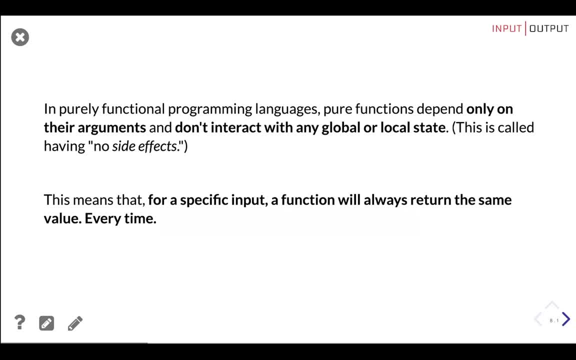 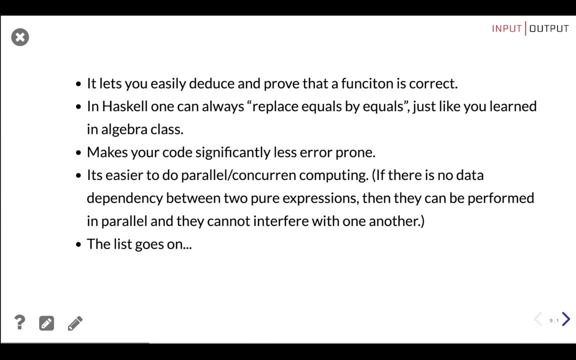 Because you are kind of constraining what you could do. But if you think about it it has some extremely convenient consequences. For example, It lets you easily deduce and prove that a function is correct. In Haskell one can always replace equals by equals. That means that if you have some definition, you can replace what the definition represents. 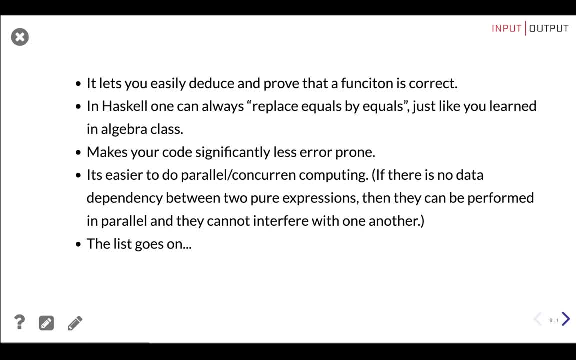 All over your code And it will still work the same. It also makes your code significantly less error-prone And it's easier to do parallel concurrent computing, Because if there is no data dependency between two pure functions, They can be performed in parallel And they will not interfere with one another. 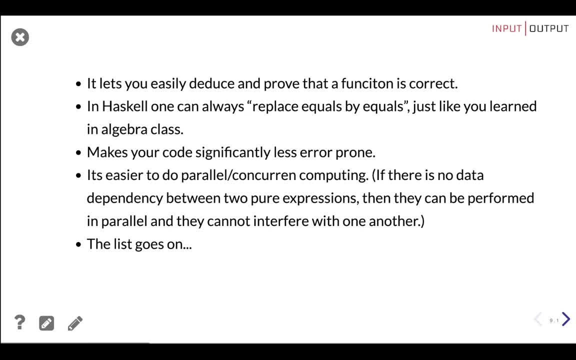 And the list goes on. Now there's a catch: If the language is completely pure, You can't interact with the outside world. Because the outside world is messy. It has errors. Not everything is perfect. Sometimes you want to read a file and the file is corrupt. Sometimes you want to get the time. 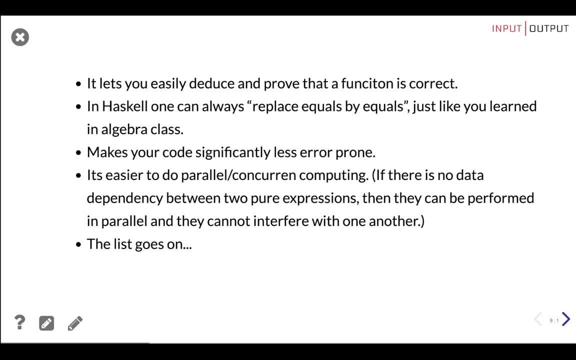 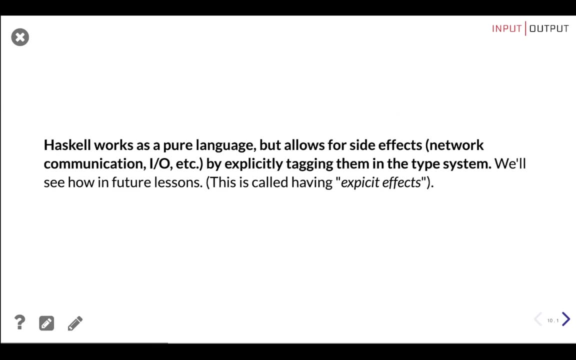 And if the same function gets the time twice, It will get different results for the same input. So you're not allowed to do that. So there's a lot of constraints around being completely pure. Haskell works as a pure language But allows for side effects Like network communication, input, output etc. 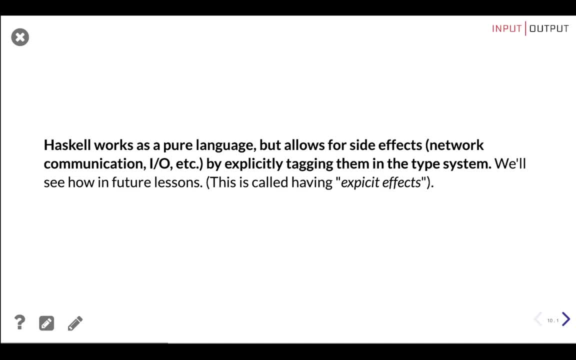 By explicitly tagging them in the type system. This is called having explicit side effects. It allows us to have the cake and eat it too, Because we can reason with our program Like a pure language, But we can also interact with the outside world And do things that are not pure. 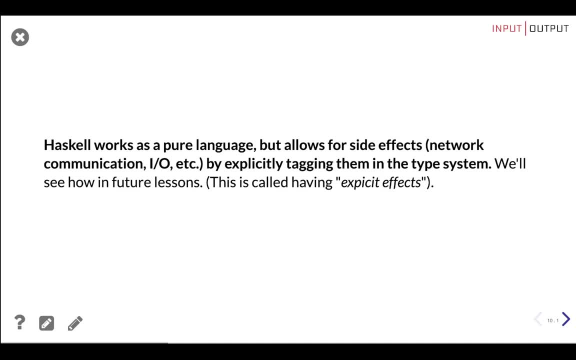 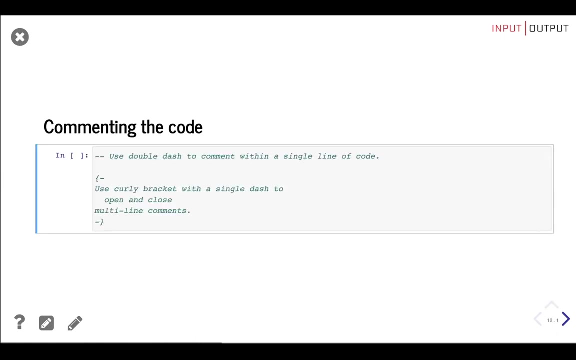 You will see concrete examples in the future, But just bear in mind that this is awesome. And before continuing with more properties, More of the theoretical side, Let's see how Haskell actually looks like. Let's see some basic syntax: Commenting the code. This is really easy: You can use double dash to comment the code. 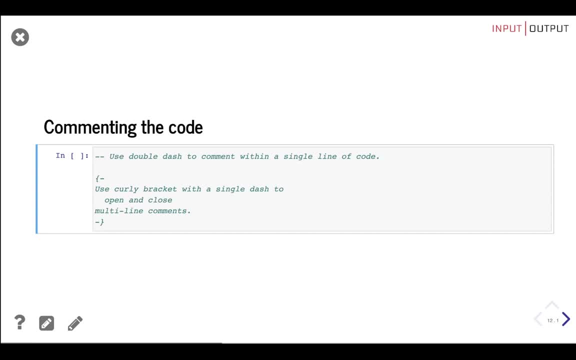 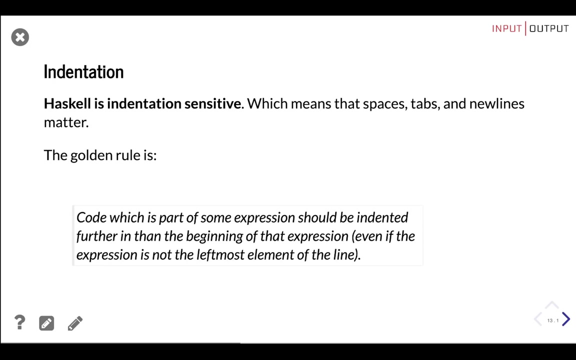 With a single line, Or you can use curly brackets with a single dash To open and close multi-line comments. Haskell is indentation sensitive, Which means that spaces, tabs and new lines matter. The golden rule here is Code which is part of some expression Should be indented further than the beginning of that expression. 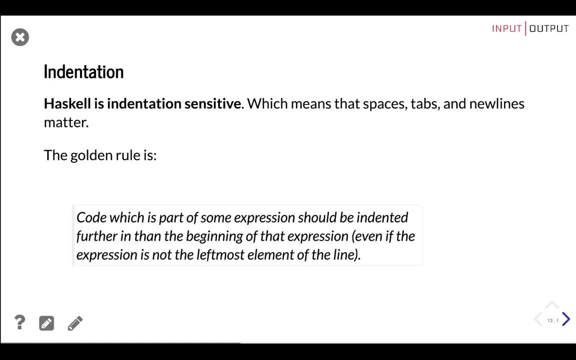 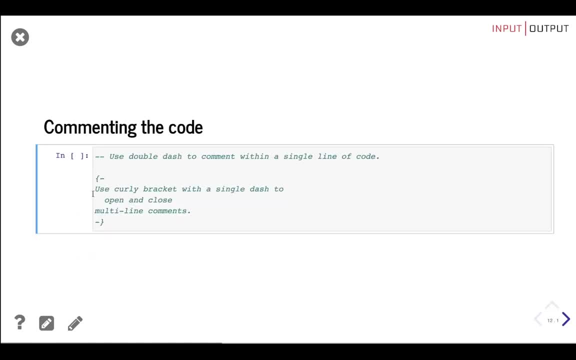 Even if that expression is not the leftmost element of the line. Let's go back to commenting the code, And if we see this code, This will be an expression. Of course it's not a valid Haskell expression, But just picture it. If this is an expression, Open and close. 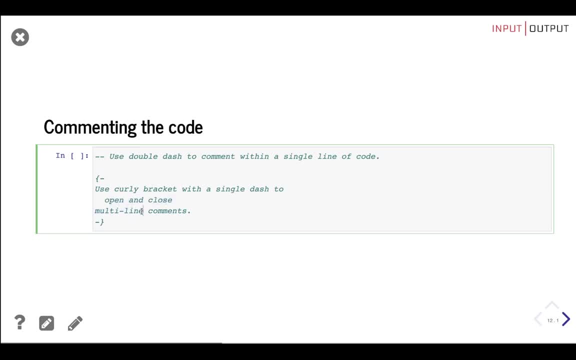 Will be part of that expression, But multi-line comments Will be not. Let's keep going. Haskell being a functional programming language Means that you're going to write a lot of functions, So that's where we'll start. This is an expression To define a function That checks if a number is greater than 18. 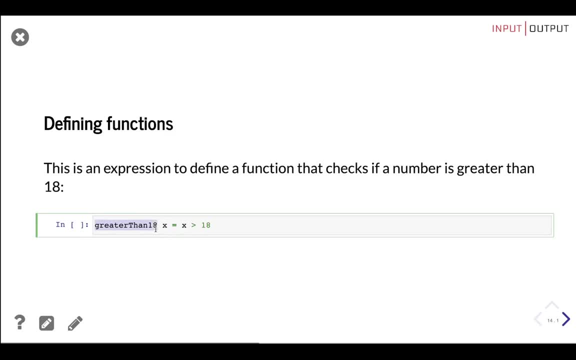 Greater than 18 is the name of the function. After the name of the function We have the parameter Of the function separated by spaces. In this case, just one parameter: x. Then the equal sign indicates The beginning of the body of the function And x greater than 18 is the body of the function. 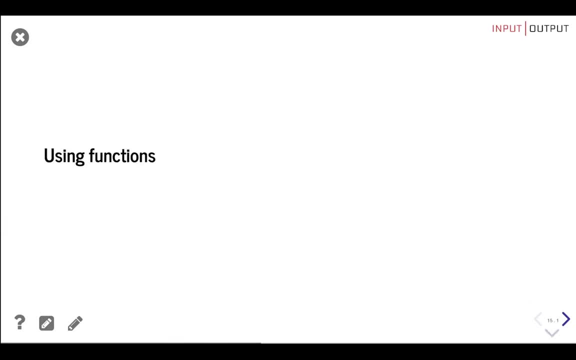 Now, To use this function, We have to provide the name of the function, Followed by the value of the parameter. In this case, 30 is bigger than 18, So it will return true, And 3 is smaller, So it will return false. Let's see a few more examples. 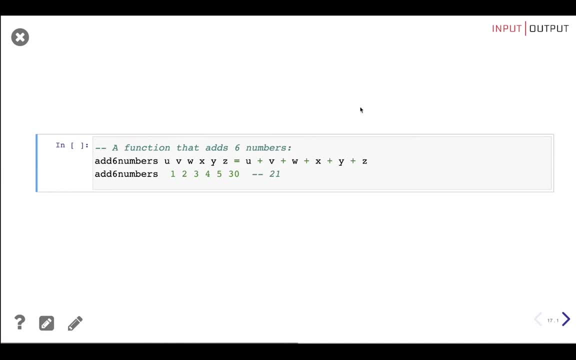 This is a function That adds six numbers. We name it, Add six numbers, Past all six parameters Separated by spaces And in the body of the function, We add them together. We use the function By providing the name And passing all the parameters Separated by spaces. We run it. 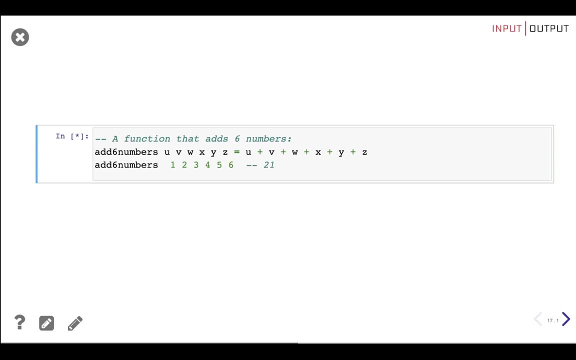 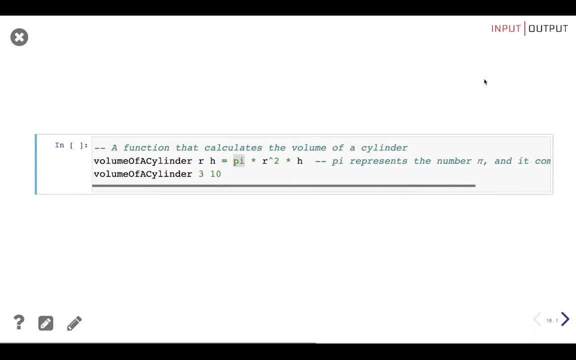 45. We can change it And run it again. 21. Ok, Now This is a function To calculate the volume Of a cylinder. We just have to provide The radius of the cylinder And the height, And in the body of the function We write the formula to calculate it. 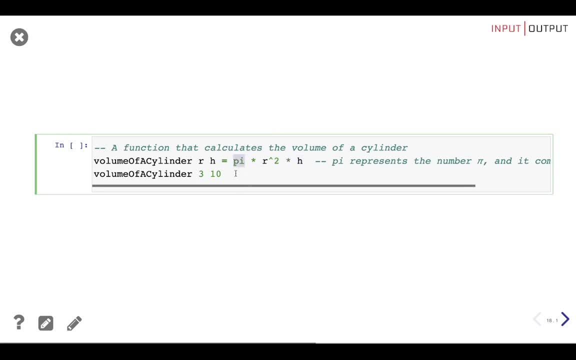 This is a constant, The pi is a constant Representing the number pi. So The volume of a cylinder Of radius 3 And height 10, It's 282 Centimeters, Meters Doesn't matter. And finally, Let's see a function That takes the temperature In Fahrenheit. 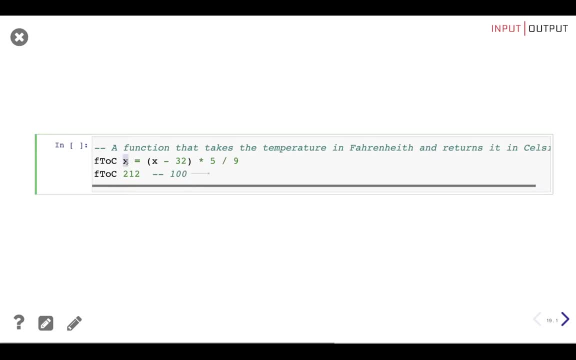 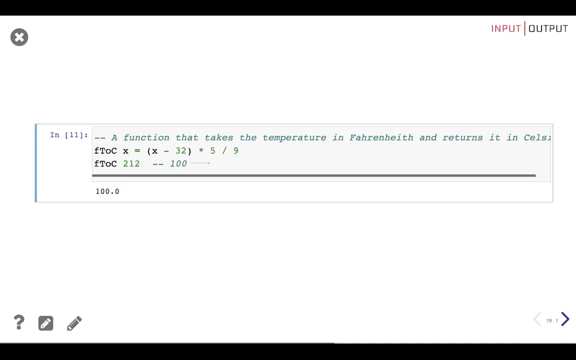 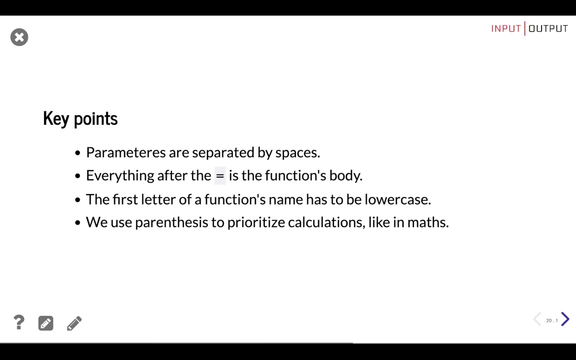 And returns it In Celsius. We have to provide The temperature In Fahrenheit. First We subtract 32 And then We multiply By 5 over 9, So 212 Fahrenheit Should be 100 Celsius. So The key points are: Parameters Are separated By spaces, Both when defining And when using. 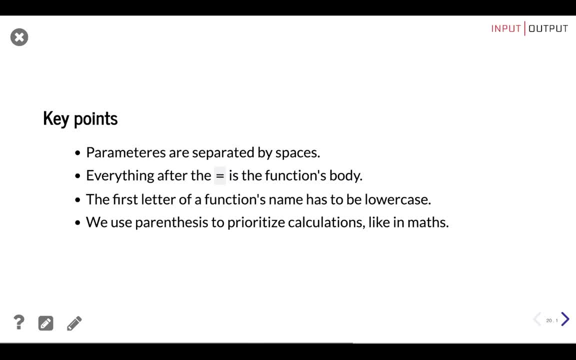 The function. Everything After The equal sign Is the function's body. It's just A single expression That represents All there is To the function. The first letter Of a function's name Has to be Lowercase And finally We use parentheses To prioritize The calculation, Like in maths. 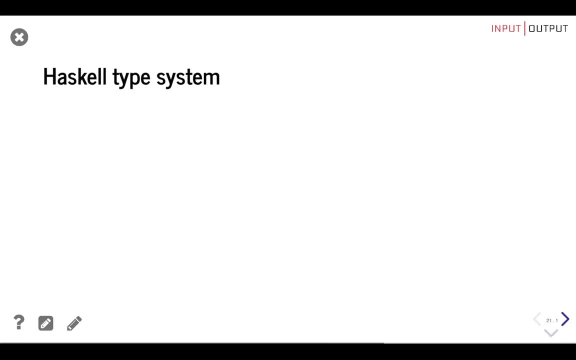 Okay, Let's go back To the theoretical side. Let's talk about The Haskell type system. You can think Of types In many different ways. You can think Of them As Attributes That constrain The values A piece of code Can have, And you can also Think of types As: 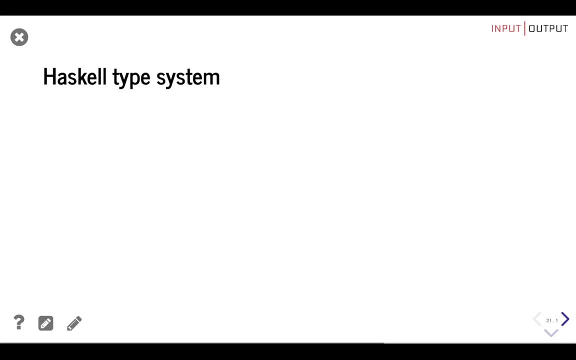 Sets That contain Values, And If a value Is contained Inside a set, The value Is of that type. So, For example, If you indicate That some data Is a number, That data Could have Any of these values. But If you try To add A letter In there Like this: 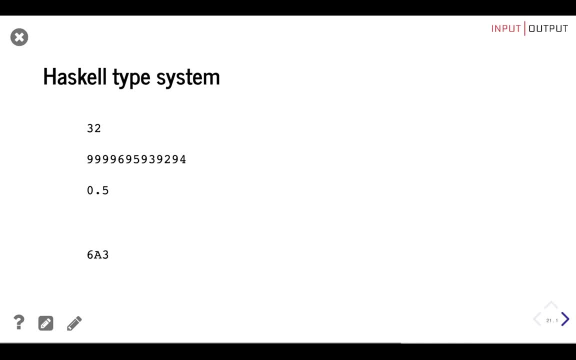 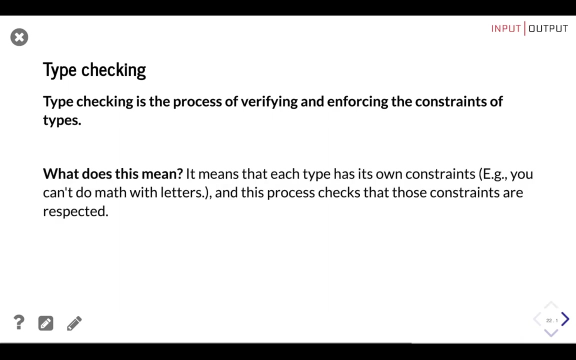 The compiler Will know, Because The compiler Knows That that's Not a number. What the compiler Did just there Is called Type checking. Type checking Is The process Of various Types By Verifying And enforcing The constraints Of types. What does this mean? Well, It means That each type 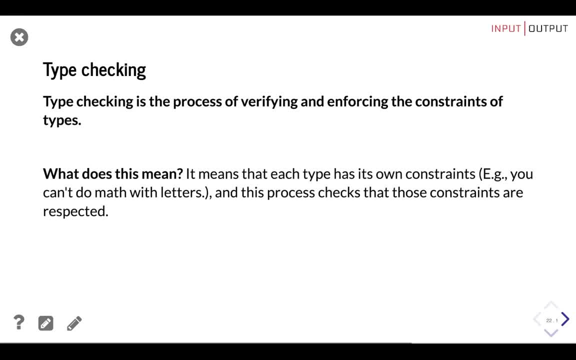 Has its own constraints. For example, You can't Do math With letters- And This process Checks That those constraints Are respected. Why would you Do this? Well, To avoid Preventable mistakes. For example, If Further along In your program You want to Do, The program Would crash. Those are 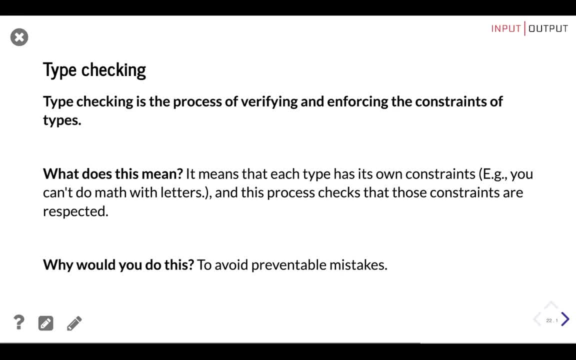 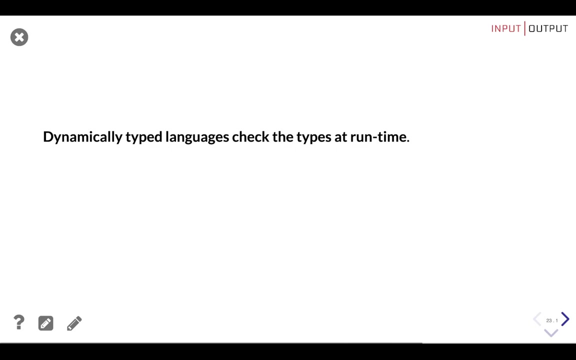 Preventable mistakes, Also called Bugs, And the compiler Helps to Avoid them. Usually, This is done Automatically, But Not all languages Do it The same way. There are Two main Distinctions Regarding When The types Are checked. You can Have Dynamically typed Languages And Types At Runtime- Runtime. 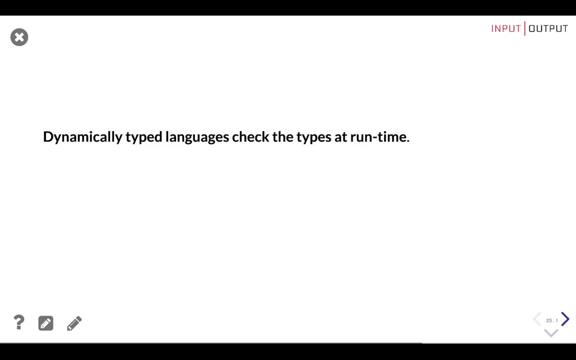 Is the Very last Thing You do With a Program. It's The stage When you Actually run Your program To test It or To use It. Common Examples Of Dynamically typed Languages Are Javascript, Python, PHP Objective- You compile The program Before running The actual Program. That leads To a. 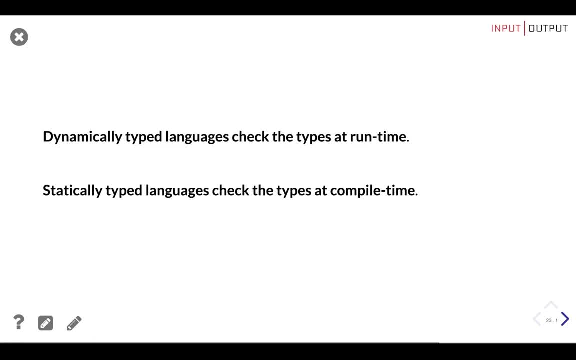 Safer and More optimized Code. Common examples Of statically typed Languages Include Java C, C++, Haskell, Haskell Type System. Haskell Is Statically Typed And In Haskell Every Java, Because Haskell's Compiler Is Very Good At Type Inference. Type Inference Allows Haskell To Invert The 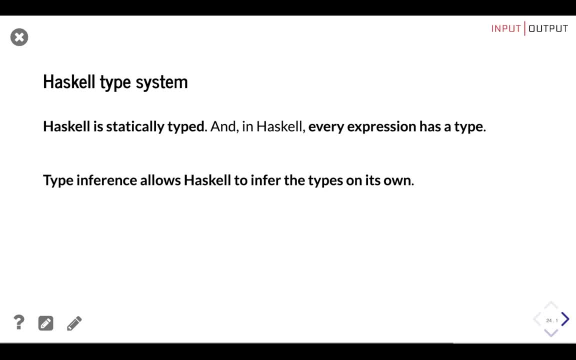 Types On Its Own. For Example, If You Write Something Like 3 Plus We Saw Before, We Never Specify That Type When We Define And Use The Previous Functions. But Haskell Could Infer The Types Of The Parameters And The Result Of The Type. It's Considered Good Practice. 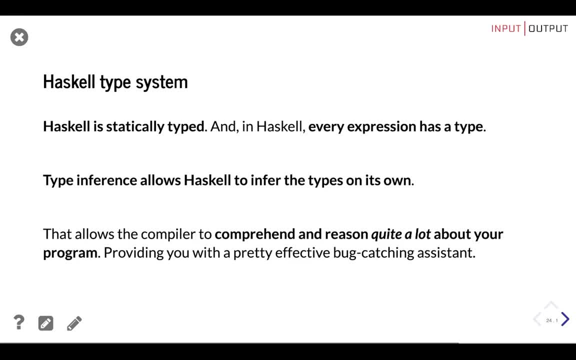 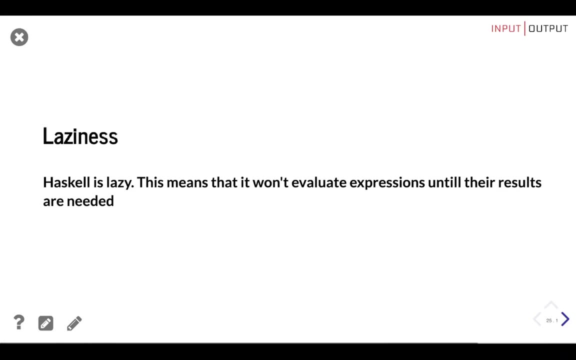 To Specify The Type Signature Of A Top Level Function To Make Your Code More Readable. Also, If The Code Is Too Ambiguous For The Function, It's Only Possible Because Of Referential Transparency, Because If You Know That The Result Of A Function Depends Only On The 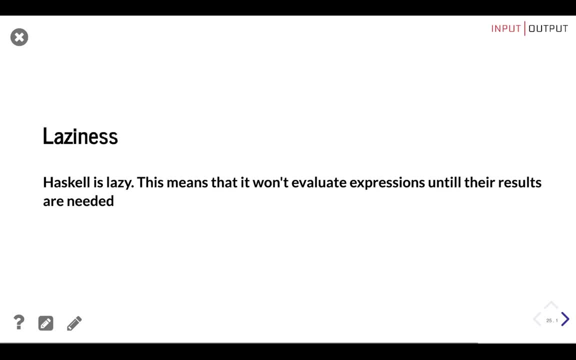 Parameters Of The Function, Then It Doesn't Make Any Sense Of The Data Structure That We Actually Need To Use. Let's See A Few Examples. So Here We Have Infinite Lists. We Can Define An Infinite That Will Take The Parameter X And It Will Take That Amount Of. 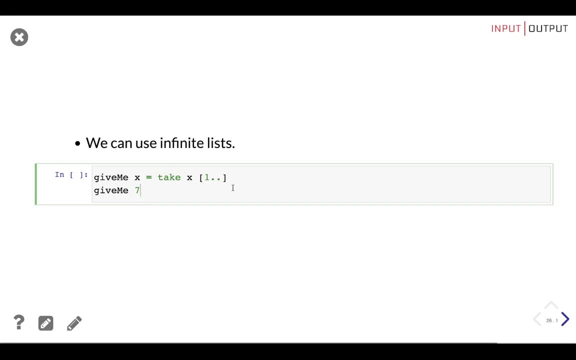 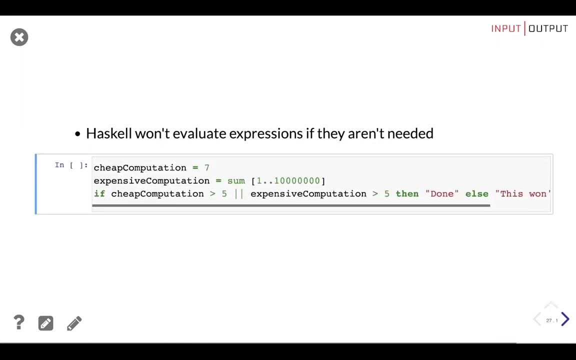 Elements From That Infinite List. Now, If We Call The Function With The Parameter Of 7, Let's See Another Example: Haskell Won't Evaluate Expressions If They Aren't Needed. So Here We Have Two Computations: Cheap Computation That Is Equal To 7 And Expensive. 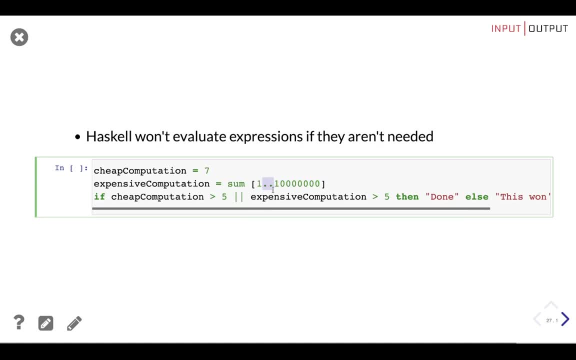 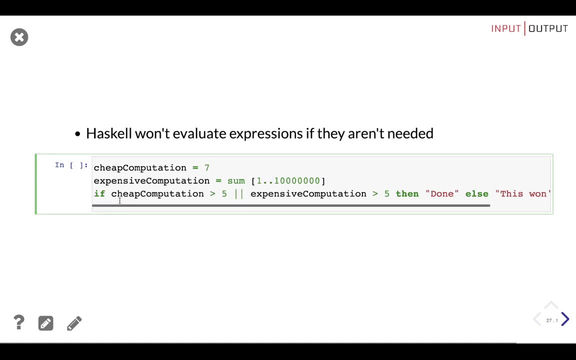 Computation. That Is The Number In Between That We Need For The Actual Computation. Now We Have A Condition: If Cheap Computation Is Bigger Than 5 Or Expensive Computation Is Bigger Than 5, Haskell Doesn't Need To Actually Calculate The Expensive. 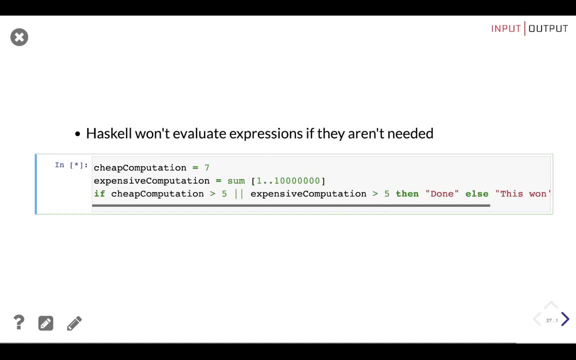 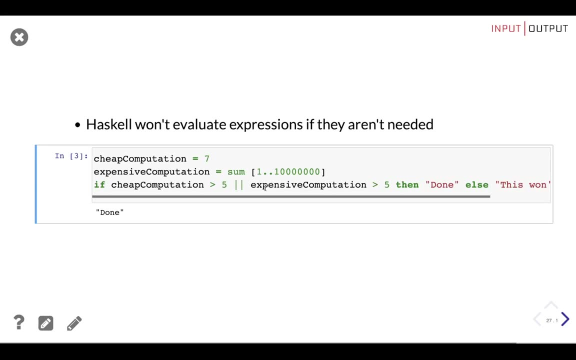 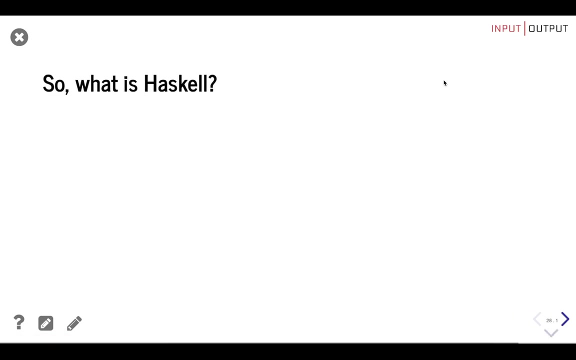 Computation This Incredible Large Sum And Check It If It's Bigger Than 5. So It Will Never Will. So If It's Bigger Than 5, Haskell Will Have To Actually Calculate Expensive Computation Because It Needs It To Compare If It's Bigger. 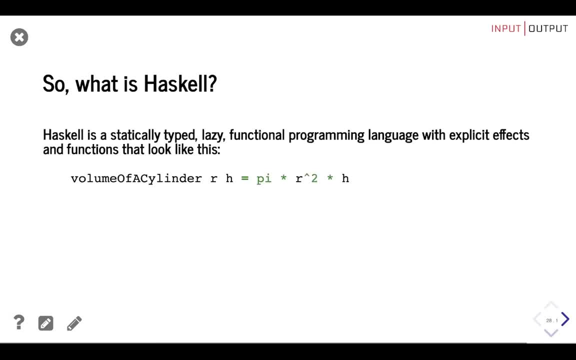 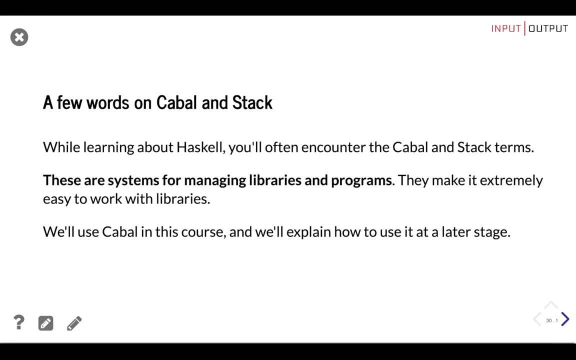 Than 5. I Won't Do This Right Now. Let's Talk About Functions, And Functions That Look Like This. Lazy And Explicit Effects Are The Most Unique Properties Of Haskell. Haskell Has Other Important Properties, Like Algebraic Data Types. To The Tools That You May Found Google Around. 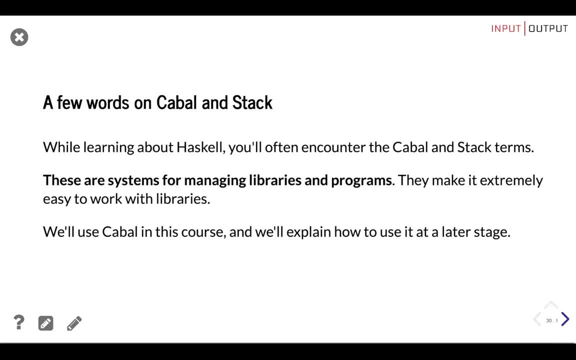 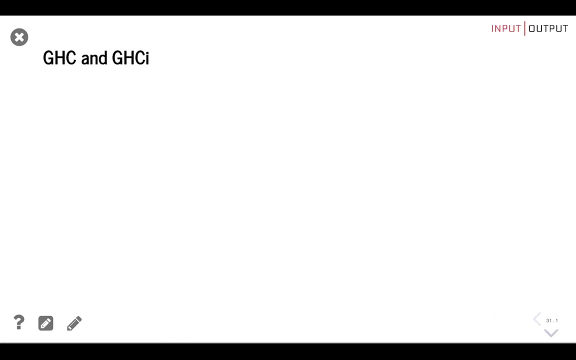 About Haskell. Let's Talk About Kaval And Stack. While Learning About Haskell, You Often Encounter The Kaval And Stack Terms, But For Now, That's All That We Are Going To Cover About Kaval And Stack, Because We Are Providing An Actual Environment With Everything Set And 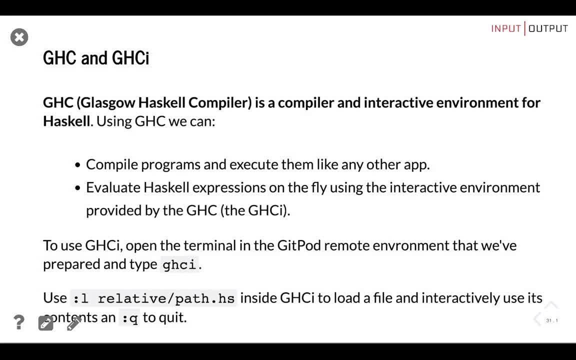 Done. And Finally, GHC And GHCI. GHC Is The Glasgow Haskell System And We Can Use The Kaval Application In Our System Or We Can Evaluate Haskell Expressions On The Fly By Using The Interactive Environment Provided By GHCI To Interactively And Use The Content. So You 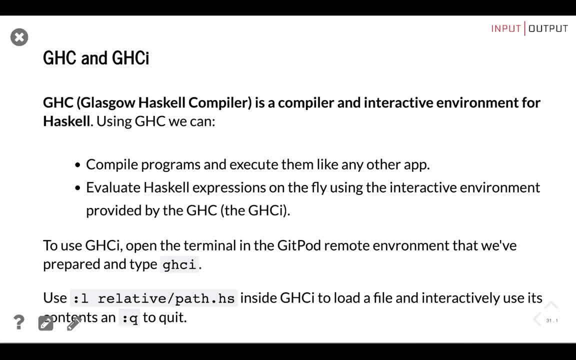 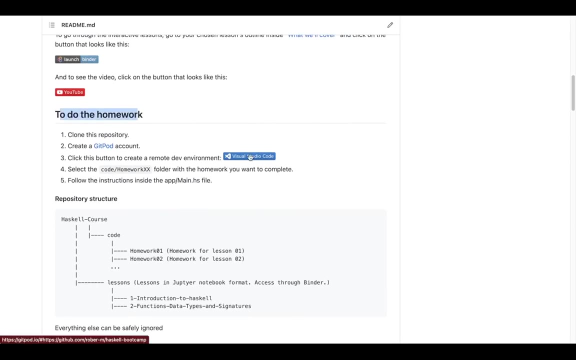 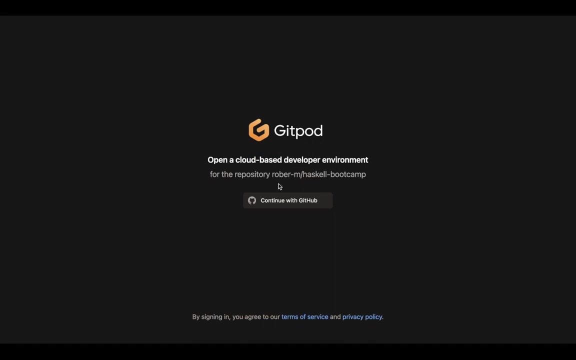 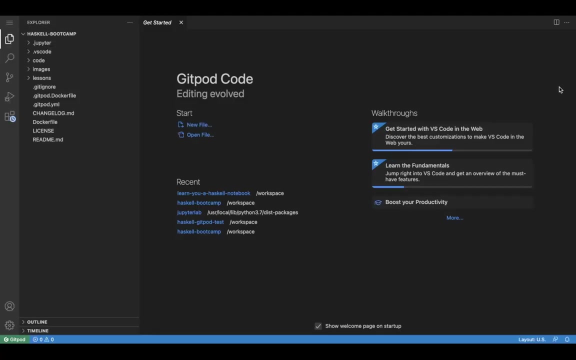 Can Create Functions, You Can Write Code In A File And Then You Can Load It To GHCI And Actually Execute The Functions And Play With The Visual Studio Code Button And It Will Open A Tab That We Ask You To Load. Okay, And We Are Ready To Go.